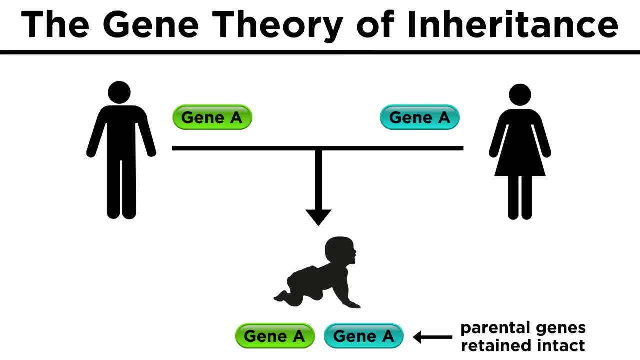 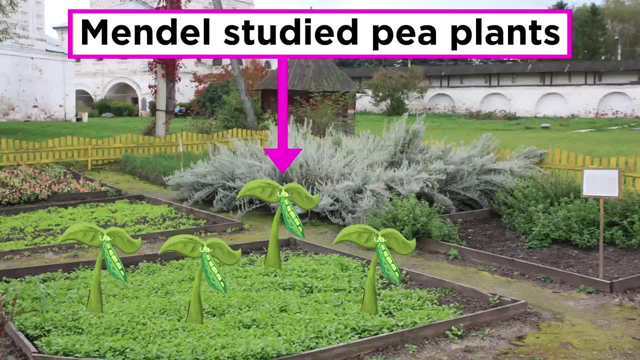 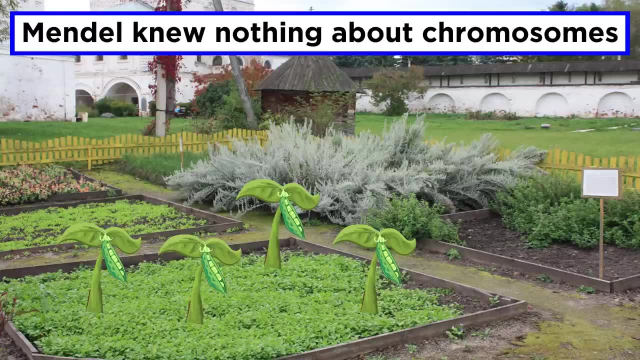 In the gene theory, each parent has a set of genes and these are retained intact in the offspring. Mendel worked for several decades with pea plants in the garden of his monastery to produce an impressive body of data to support the gene theory, all of which was done decades. 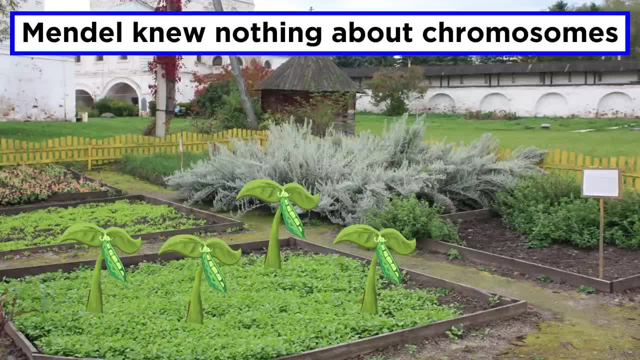 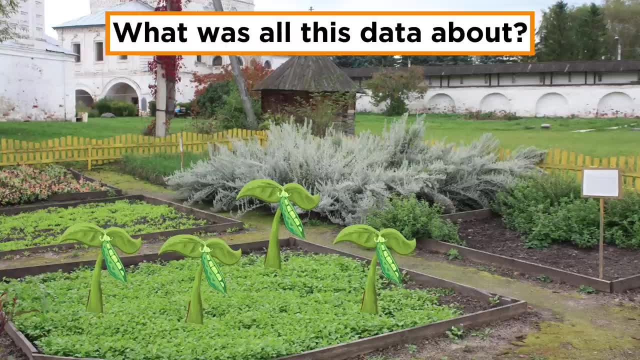 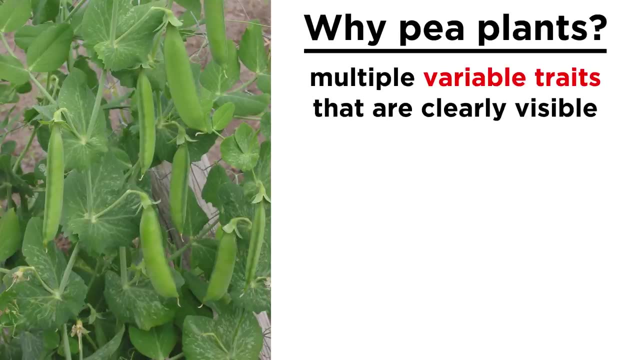 before chromosomes were observed and understood. We will discuss the methods Mendel used to breed the pea plants and the conclusions he was able to derive from them. First of all, why peas? Well, the pea plant has a number of visible traits that can vary, so results are easy. 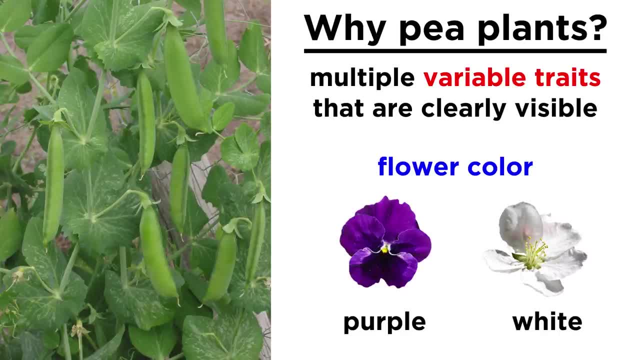 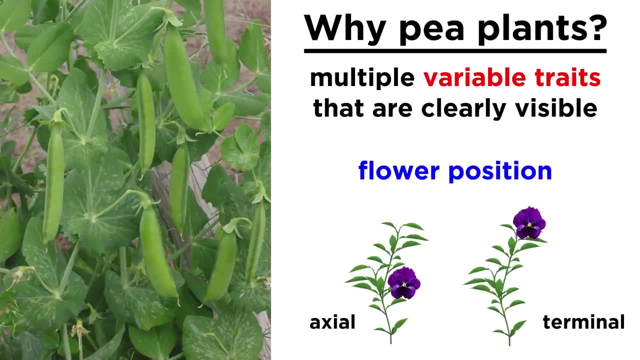 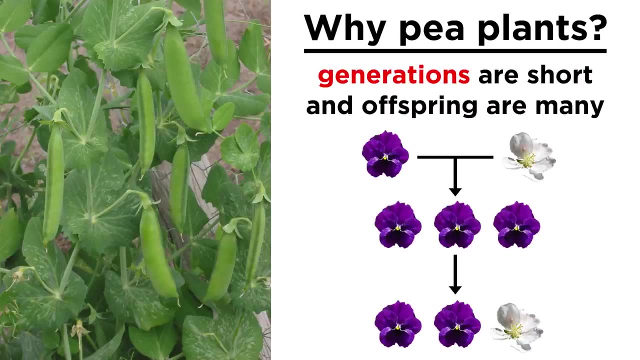 to observe. These are things like flower colors. These are things like flower colors: Seed color and shape, pod color and shape, flower position and stem length. Generations of the pea plant are short and the offspring are many, so data is easy to. 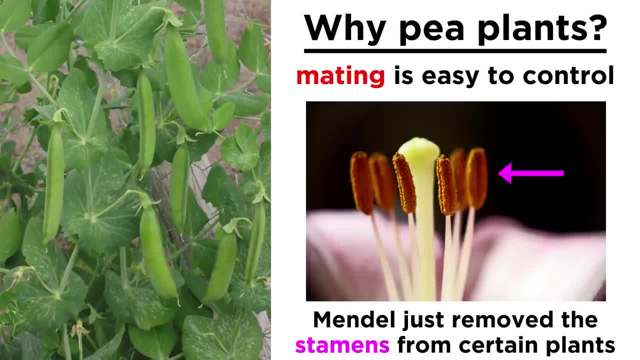 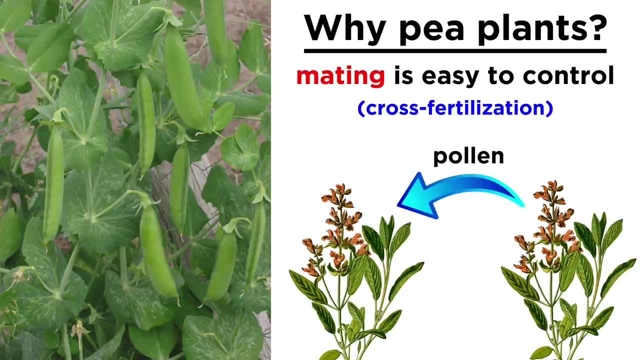 gather And Mendel could easily control mating by removing the stamens, the male fertilizing organs that produce pollen, from a particular set of plants. then he could deliberately cross-fertilize with pollen. This means he had complete control over which plants were mating with which other plants. 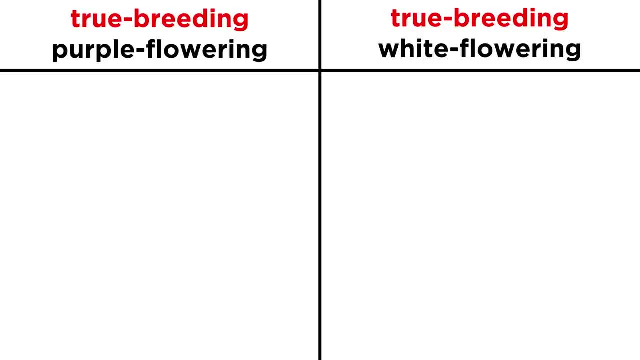 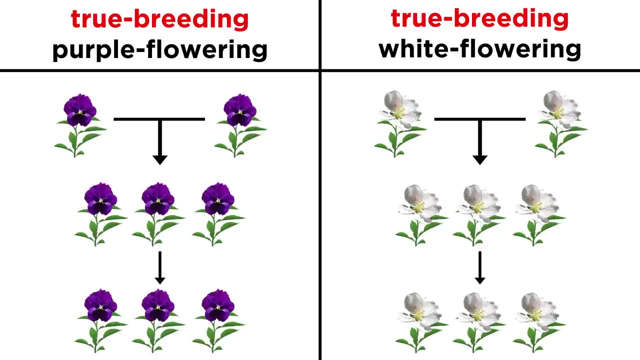 Some plants were true breeding with respect to a particular trait, meaning that some plants with purple flowers, when self-fertilizing, gave generation after generation of entirely purple flowering plants. The same goes for the plants with white flowers, So this meant he could breed with purple flowers. 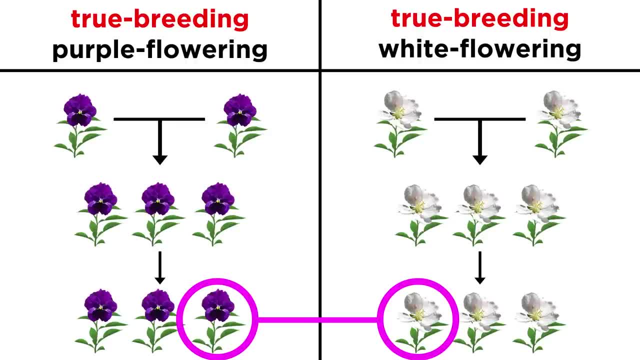 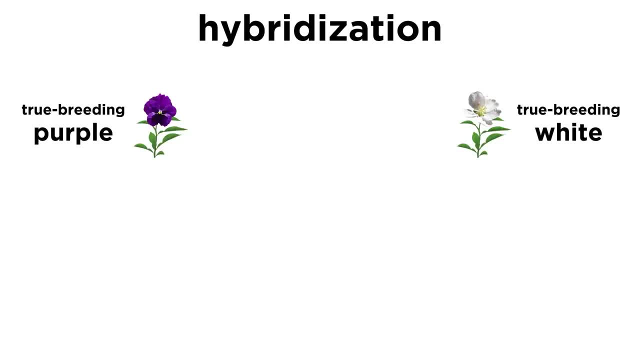 This meant he could breed true-breeding white flowering plants with true-breeding purple flowering plants and see what happens. This kind of process is called hybridization, and we can call the two true-breeding plants the parental generation, while the offspring will be referred to as the F1 generation. 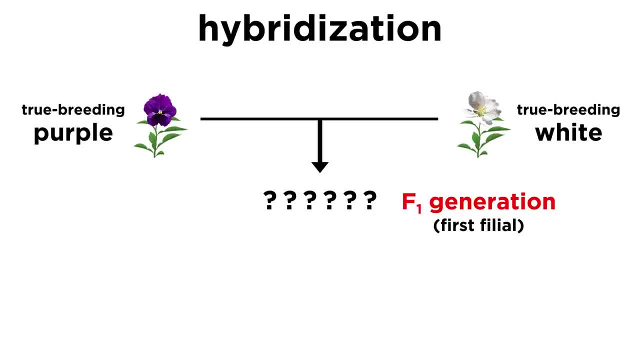 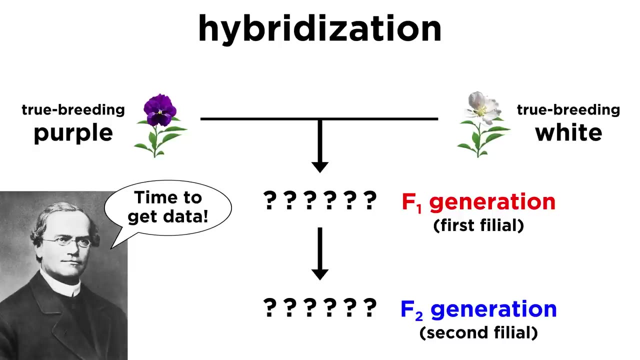 or the first filial generation from the Latin word for sun. If these F1 plants are allowed to reproduce further, we get the F2.. Mendel did experiment after experiment with different kinds of pea plants following the traits expressed or phenotypes, up to the F2 generation. 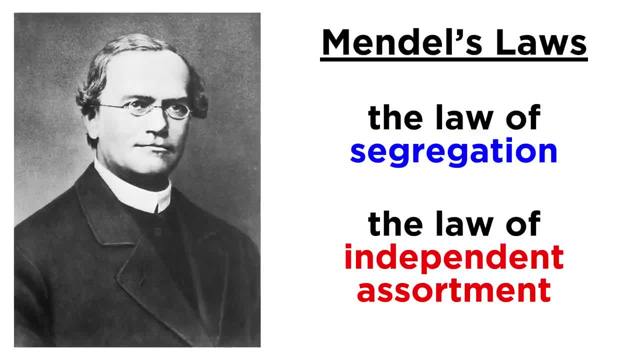 From this mountain of data, he developed two fundamental laws of genetics. These are the law of segregation and the law of independent assortment. To see how these laws were derived, let's examine one of his experiments. Let's say purple flowering and blue flowering are the same. 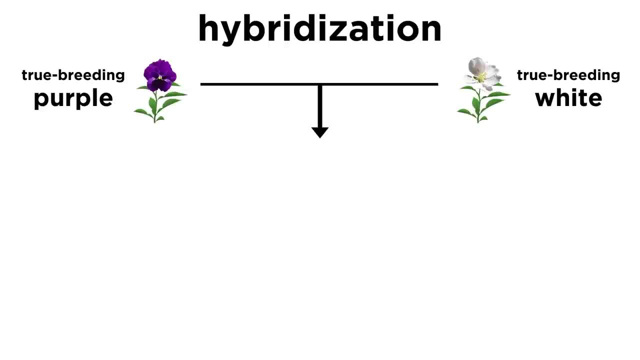 Let's say purple flowering and blue flowering are the same. Let's say purple flowering and blue flowering are the same. Let's say purple flowering and white flowering plants are hybridized. We would find that the F1 generation is entirely purple. No white, no pink, just all purple. 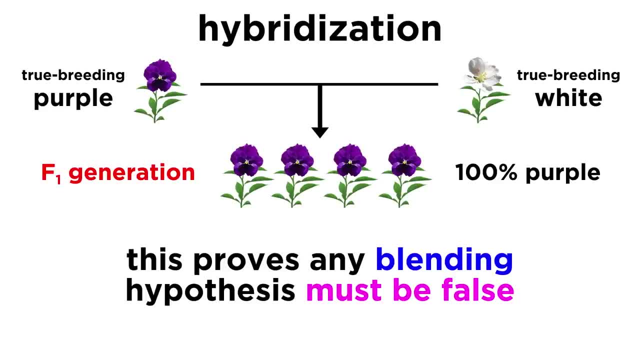 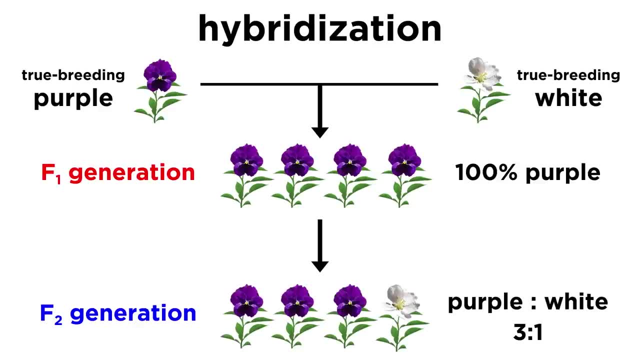 This experiment alone proves that any kind of blending hypothesis must be false. But even more perplexing is that if the F1 generation is allowed to self-pollinate, the F2 generation gives plants that are both purple and white in roughly a three to one ratio. 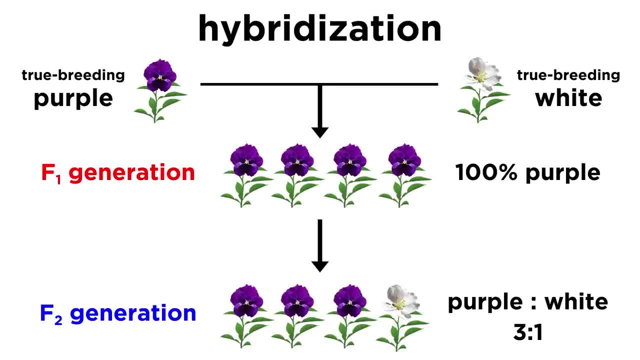 This strongly supports what we now refer to as the gene theory, because it means that somewhere in the F1 plants there must have been some kind of information pertaining to white flowers that was not lost and was expressed later with the F2 plants. 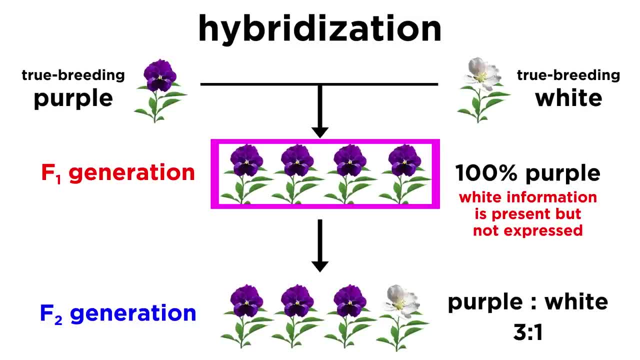 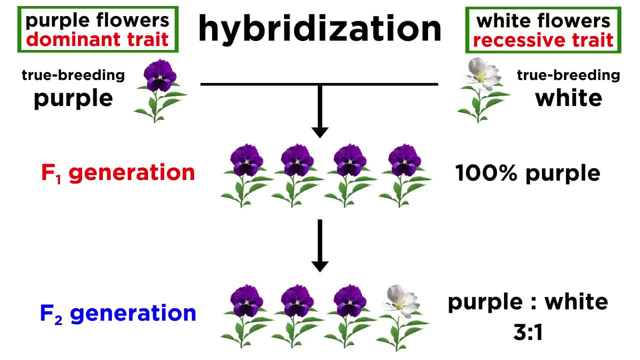 This white flowering gene must simply have been hidden or silenced in the F1 plants. We can therefore refer to purple flowers as the dominant trait and white flowers as the recessive trait. This combination of dominant and recessive traits is called the white flowering gene. 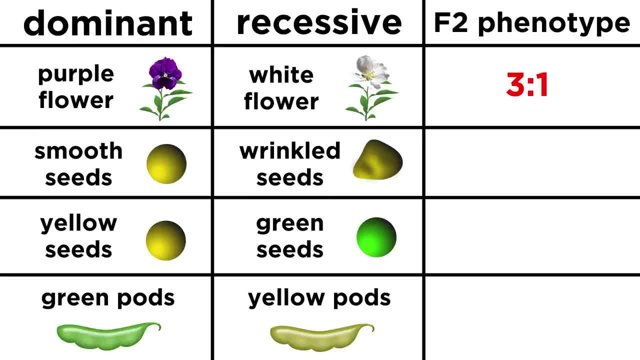 Each trait was observed for many other aspects of the plant, and precisely the same three to one ratio was observed when examining the phenotypes in the F2 generation for smooth versus wrinkled seeds, yellow versus green seeds, green versus yellow pods, and so forth. 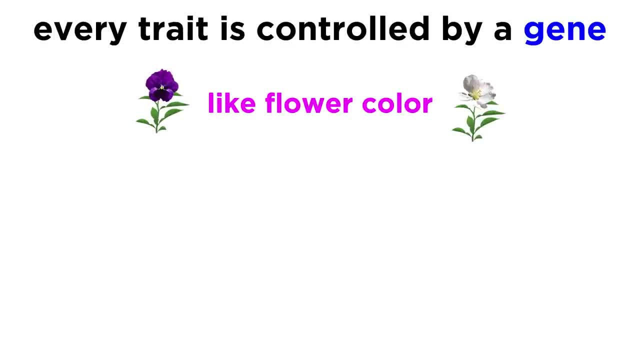 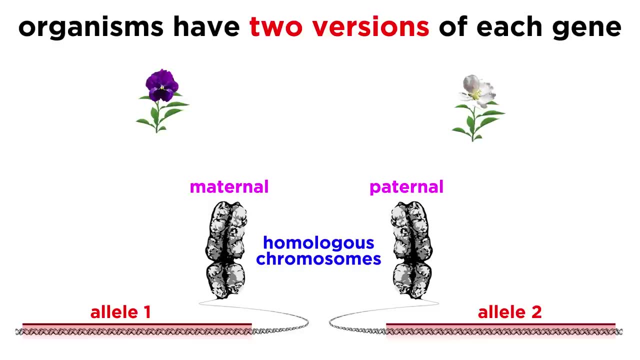 The reason for this is that each trait corresponds to a particular gene, like a gene for flower color, But each gene has two versions or alleles in the genome, Because the gene is found on two homologous chromosomes, one from each parent. 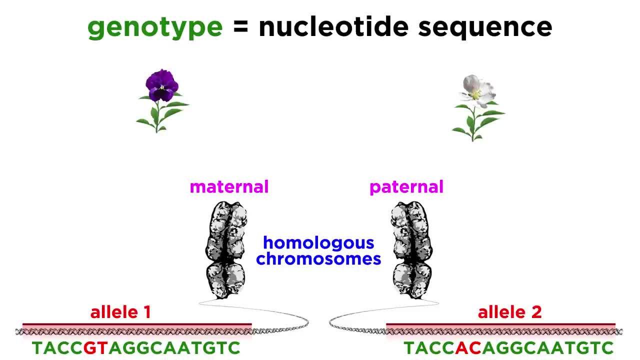 These two alleles can be of a different genotype, meaning that the sequence of nucleotides are different, and this can lead to different phenotypes when expressed like the two different colors that are visible on the flower. Although Mendel didn't know anything about DNA, he was still able to decipher this concept. 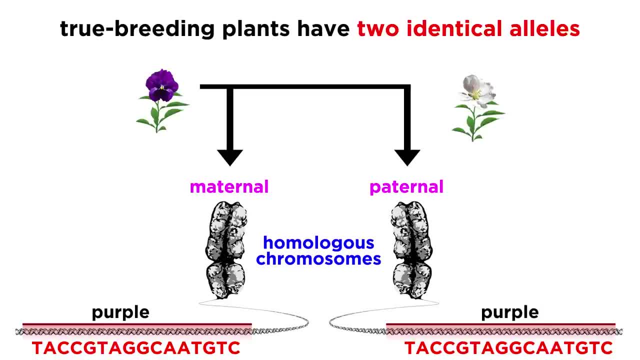 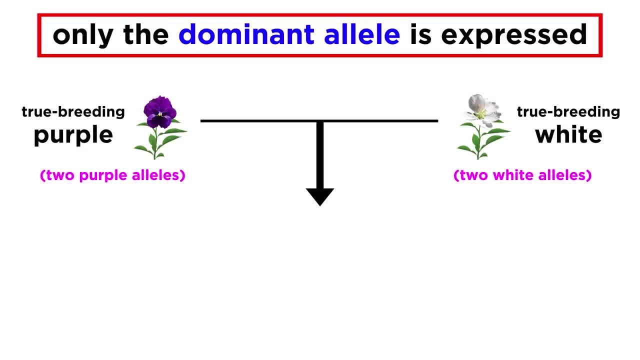 of two alleles per trait. True breeding plants must have identical alleles for a particular trait. but when he performed the hybridization, he realized that one allele was dominant in that it was expressed, while the other was recessive and stayed dormant. In this case, when purple and white are hybridized, the F1 generation is all purple, so purple. 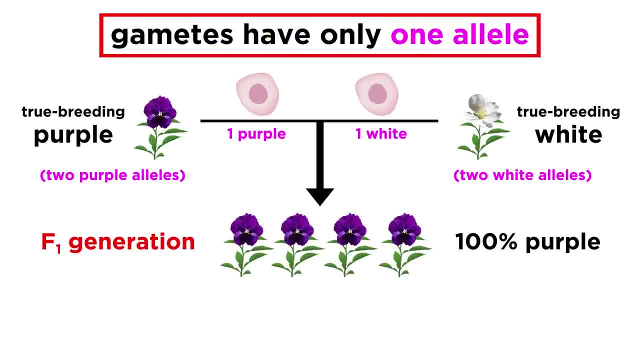 must be dominant. He even realized that each gamete must have only one allele. So that's why he said that all alleles are dominant. In other words, the F1 generation is all purple, so purple must be dominant. He even realized that each gamete must have only one allele. 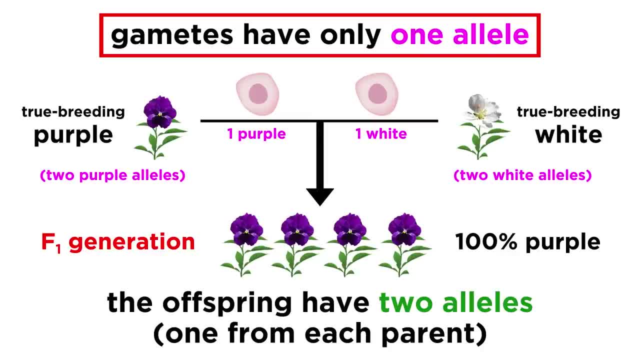 He even realized that each gamete must have only one allele, such that when each plant is fertilized, one of any of the possible combinations of alleles will result. This is the law of segregation. We now understand this is true because we have learned about meiosis and the haploid. 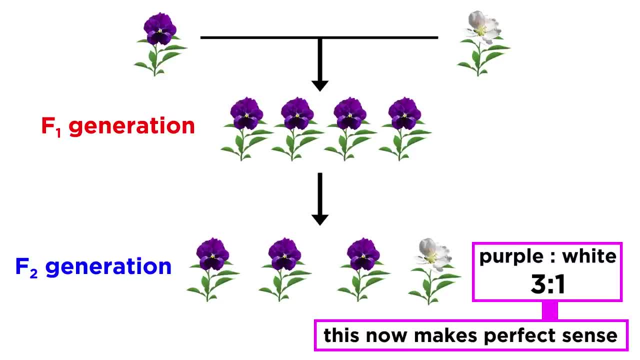 daughter cells that result. In this way, Mendel was able to explain the phenotypes in the F2 generation by rationalizing that true breeding purples have two purple alleles and true breeding whites have two white alleles. so when the sperm from one fertilizes the egg from the other, all of 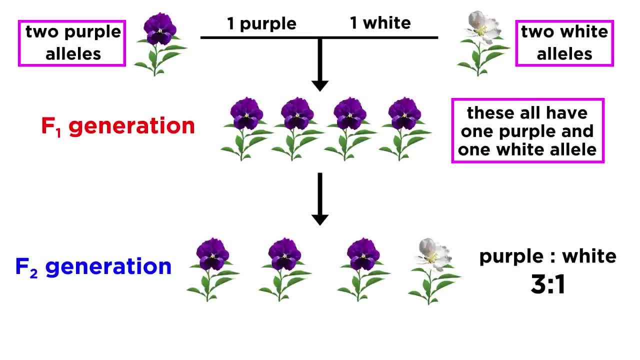 the resulting plants in the F1 generation must have one of each allele, Because purple is dominant. they are all purple. but when the F1 generation produces its own gametes, some will be purple and some will be white. so when they self-fertilize there, 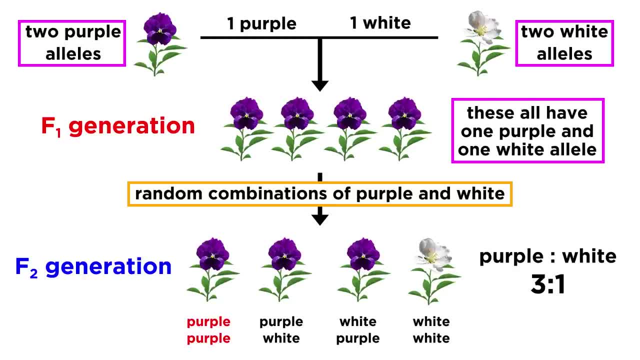 are four possible combinations, and those are: purple and purple, purple and white, white and purple or white and purple, Since purple is present in three of those. that explains the three to one ratio, given that only a plant with two recessive white alleles will appear white. 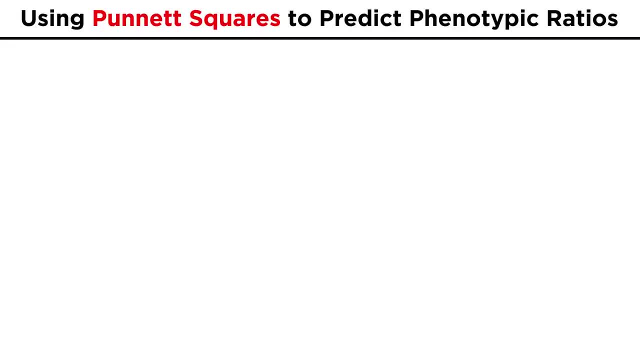 This kind of logic can be displayed using Punnett squares. For these we make a grid and along the top boxes we place the alleles for one plant. If we are allowing the F1 generation to reproduce, all of those have one purple allele. 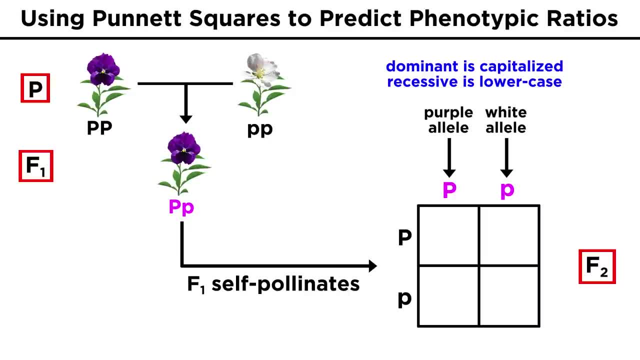 This is called a purple allele, which we can symbolize with a capital P, since we capitalize the dominant allele and the white allele will be a lowercase P as it is recessive. The other plant will have its alleles to the left of the boxes. 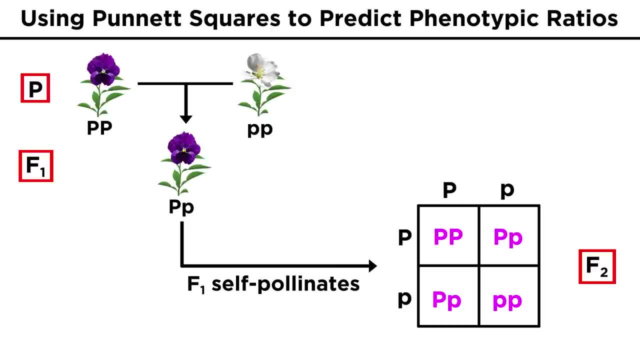 Then we just populate the boxes to form all the possible pairing combinations. Dominant alleles are listed first and there is the distribution, just as we described before, with a three to one ratio of purple to white in the F2.. two generation: When an organism has identical alleles for a particular gene, it is said to be homozygous. 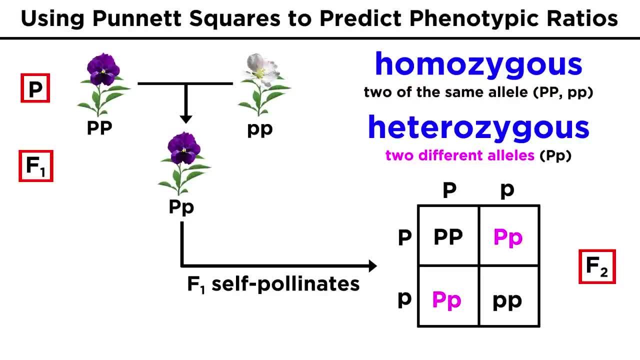 for that gene If it has one of each allele, we call it heterozygous. As we can see, homozygous dominant and heterozygous both result in the dominant phenotype Only homozygous recessive results in the recessive phenotype being visible in the plant. 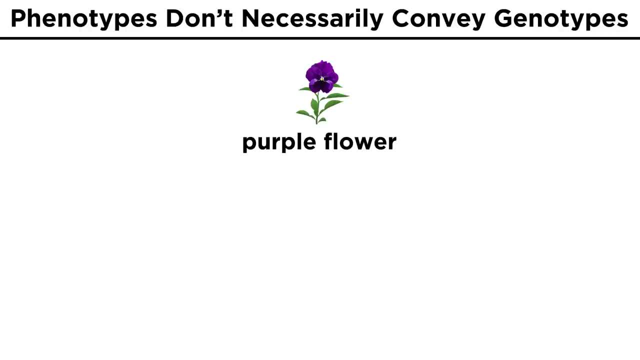 For this reason, we must understand that observing the phenotype that is visible for a particular trait in an organism does not tell us with certainty what genotype is present, as multiple genotypes result in the same phenotype. However, we can breed this organism with another organism that has a known genotype for that. 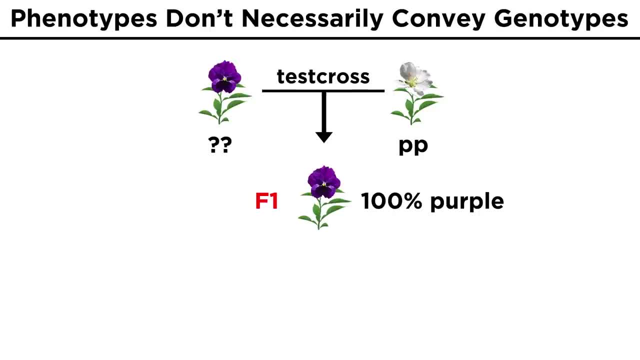 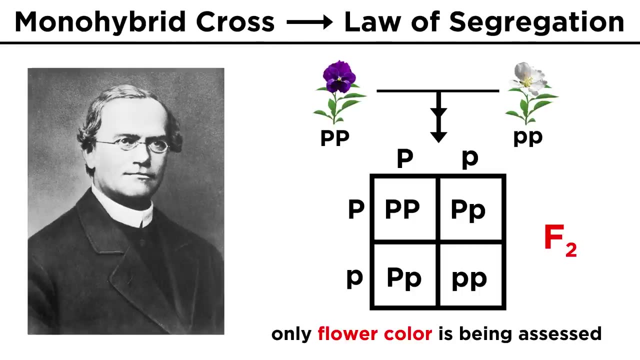 trait and analyze the phenotypic distribution in the resulting generation to decipher what the unknown genotype is. This is what the genotype must be. When Mendel discovered the law of segregation, he was looking at one trait at a time, which we would call a monohybrid cross. 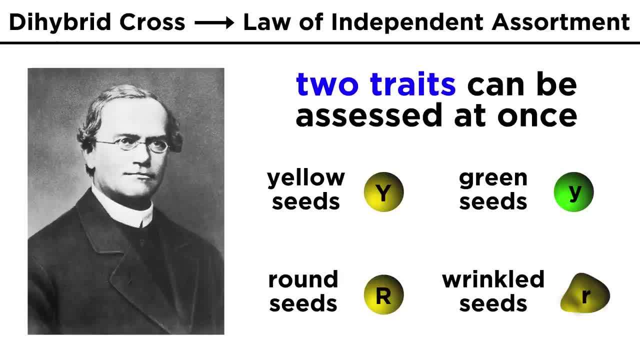 But when he started looking at two traits at the same time, he discovered the law of independent assortment. He knew that the seeds of the pea plant could be either yellow or green, with yellow being dominant, and they could either be round or wrinkled, with round being dominant. 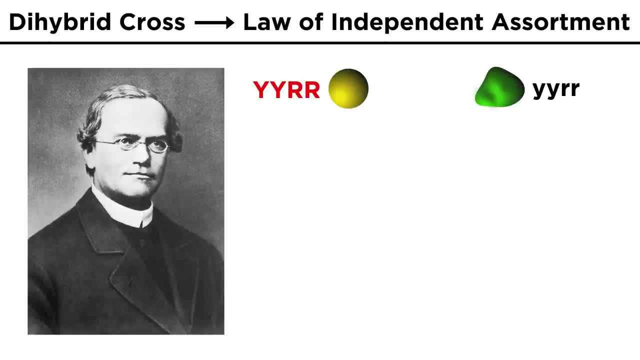 He took true breeding plants with round yellow seeds and crossed them with true breeding plants with wrinkled green seeds, performing a dihybrid cross. As we would expect, all the plants in the F1 generation end up heterozygous for both. 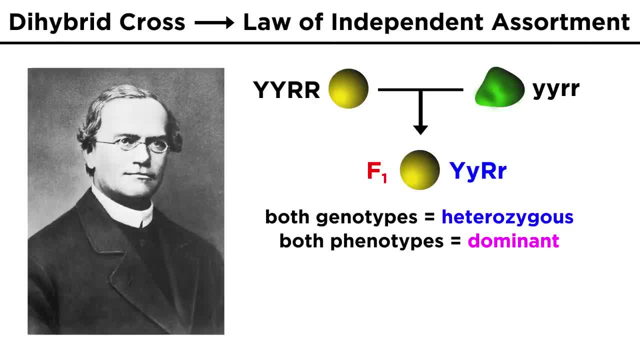 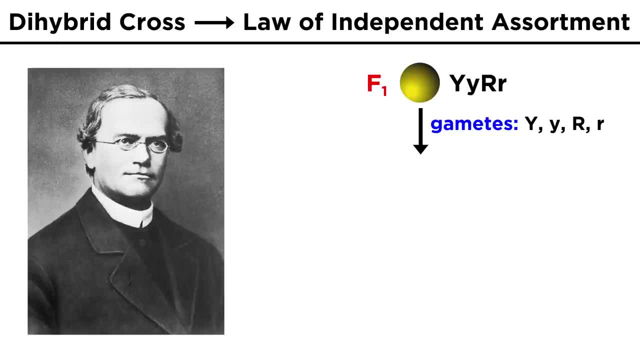 traits, thus exhibiting the dominant phenotype for both traits. But because we are examining two traits at once, there are now four possible combinations of alleles producing a monohybrid cross. The monohybrid cross is produced in the gametes of the F1 plants. 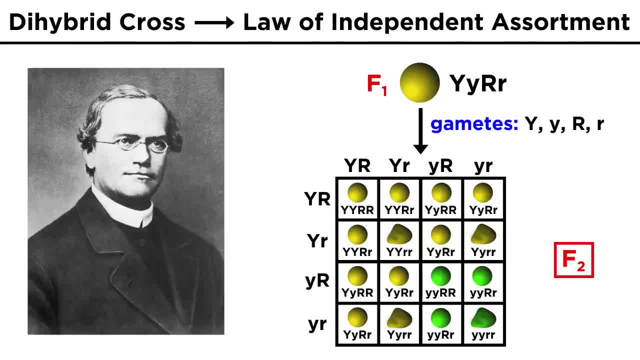 If these plants reproduce, we end up with a variety of possible genotypes for the F2 plants, because the Punnett square must involve all possible combinations of all possible gametes from two different plants. The phenotypic distribution for a dihybrid cross will always be nine to three to three. 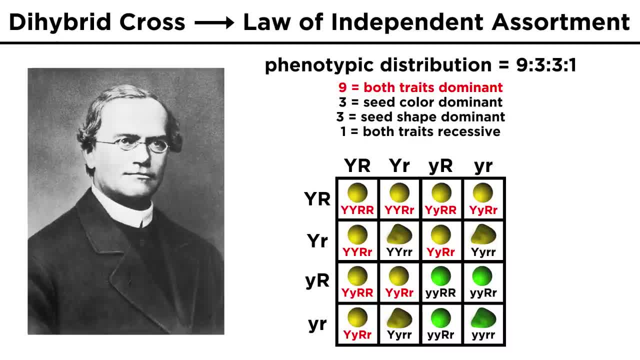 to one, where nine represents the proportion of the F2 generation that will exhibit the dominant phenotype for both traits. Three represents the proportion that will show dominant for one and recessive for the other. The other three is for the reverse situation and the one is for the ones that will be recessive. 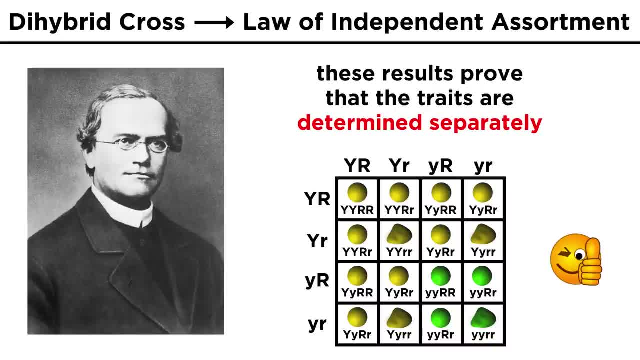 for both. These results are significant because they show that each trait is determined individually. Just because the F1 generation was heterozygous, it doesn't mean that the F2 will be The alleles for each trait separate after the F2 generation. 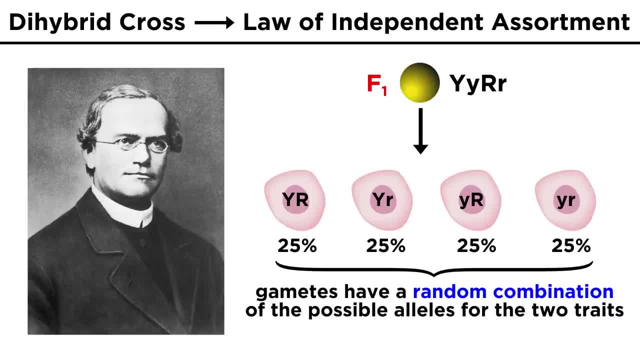 The alleles for each trait, separate after the F2 generation. The alleles for each trait, separate after the F2 generation. They are only at random during gamete formation, thus demonstrating the law of independent assortment and also demonstrating that the combination of alleles that occur in any given organism. 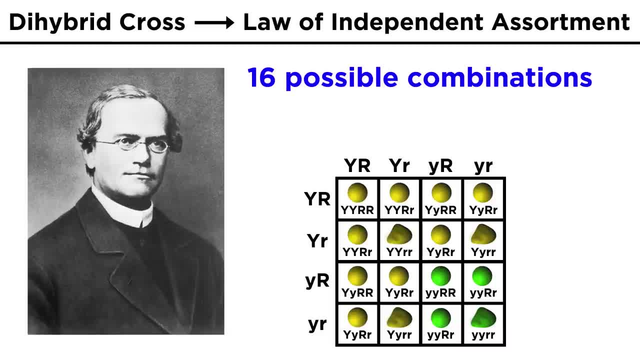 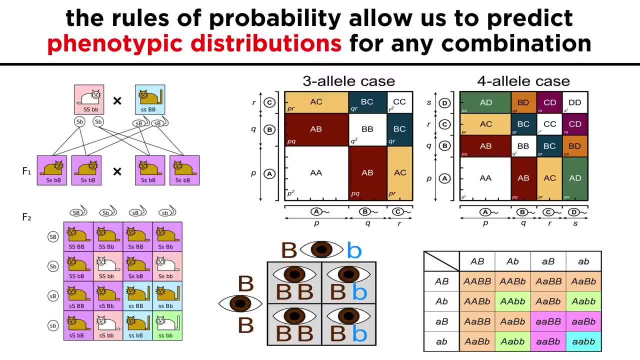 is determined entirely by probability. Sixteen possible combinations, one in sixteen chance for each one, so roughly one in every sixteen plants will exhibit a particular genotype. Because of this mathematical reliability, we can use the rules of probability to closely predict phenotypic distributions for more complicated combinations. 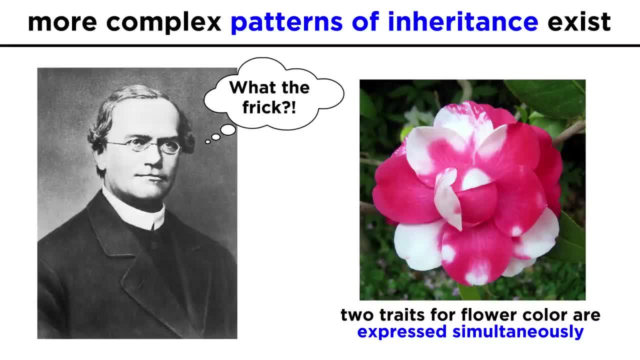 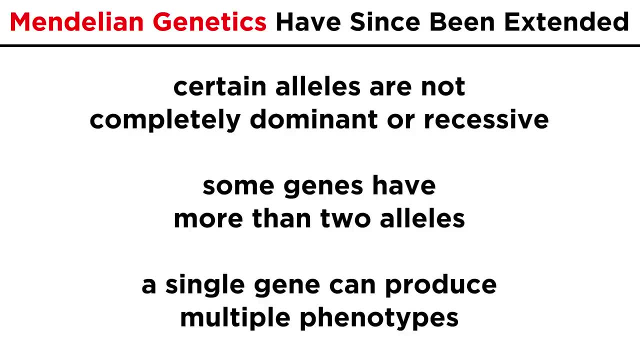 Not all patterns of inheritance are this simple. unfortunately, and as impressive as Mendel's experiments were, he could not explain certain observations, But since his time we have extended Mendelian genetics to explain these observations as well, as we now understand that certain alleles are not completely dominant or recessive. 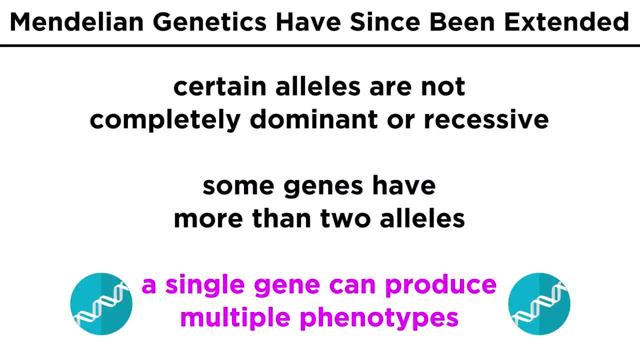 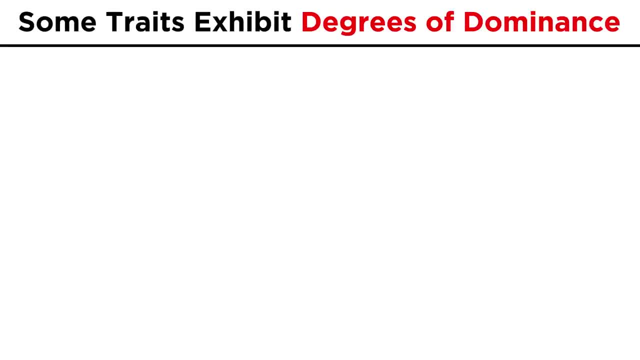 Some genes have more than two alleles and a single gene can sometimes produce multiple phenotypes. For example, there are degrees of dominance. With everything so far, we have been discussing complete dominance, where the dominant allele is expressed, whether the genotype is homozygous or heterozygous, and there is no difference.